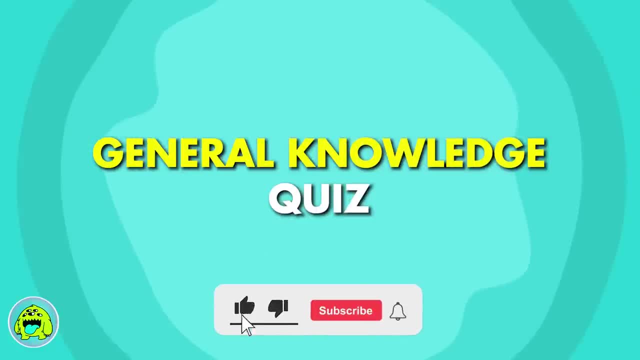 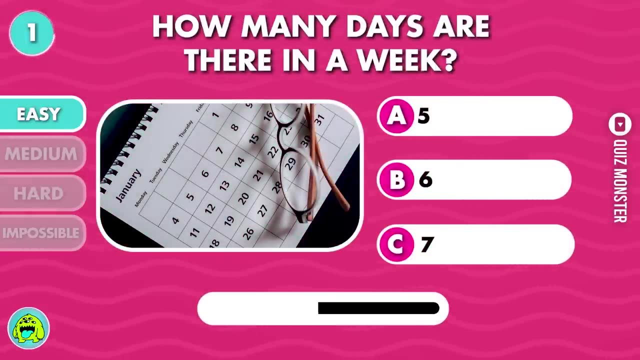 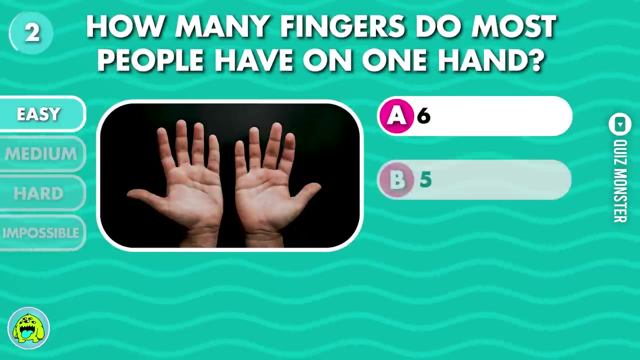 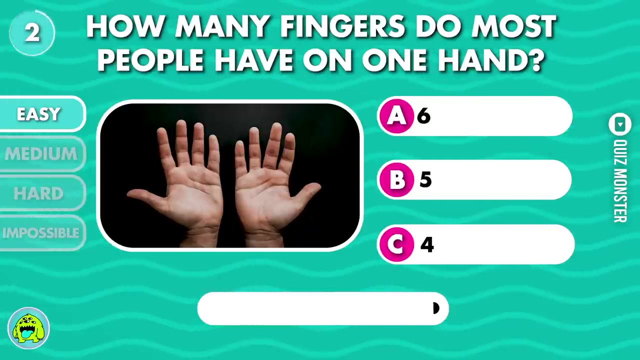 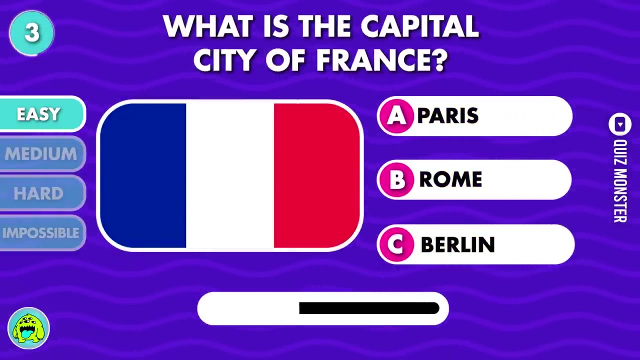 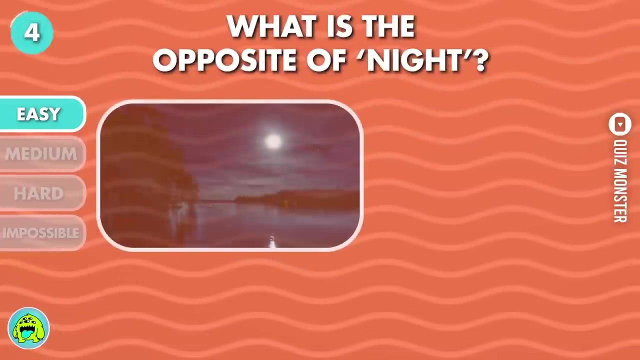 Hey Monsters, Get ready for a fun general knowledge quiz. Let's go. How many days are there in a week? Seven. How many fingers do most people have on one hand? Five. What is the capital city of France, Paris? What is the opposite of night? 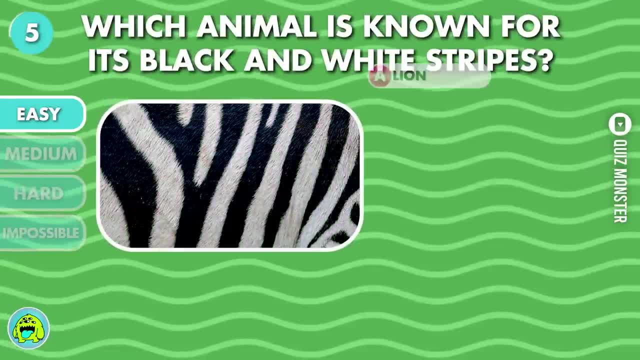 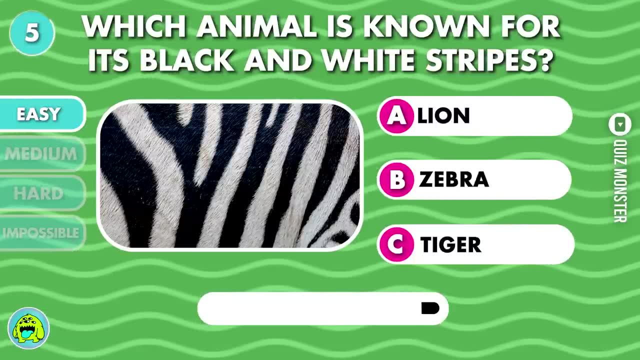 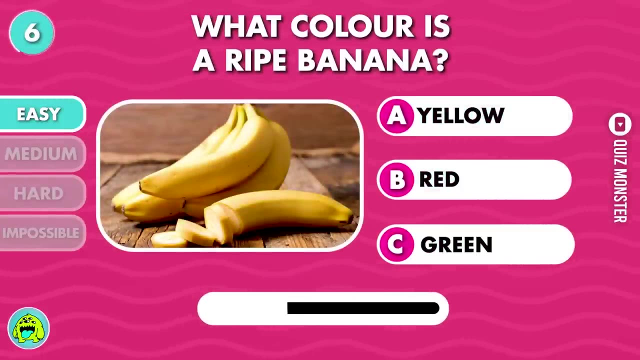 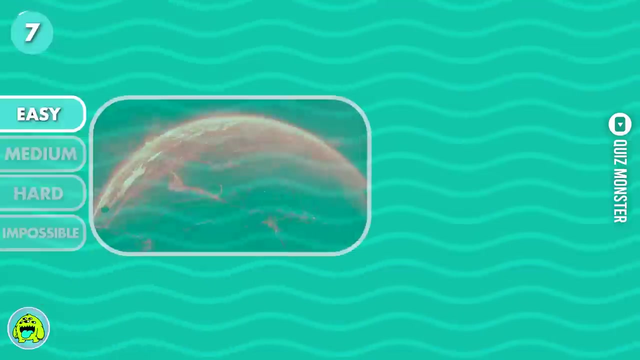 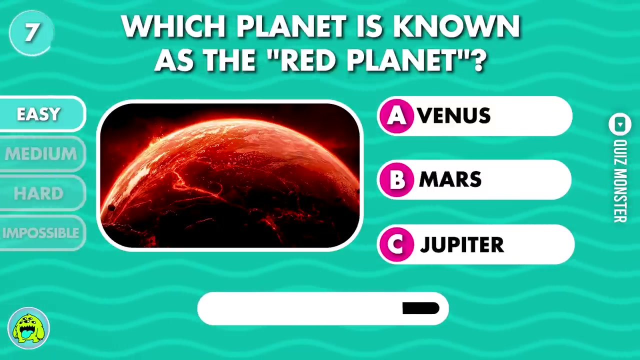 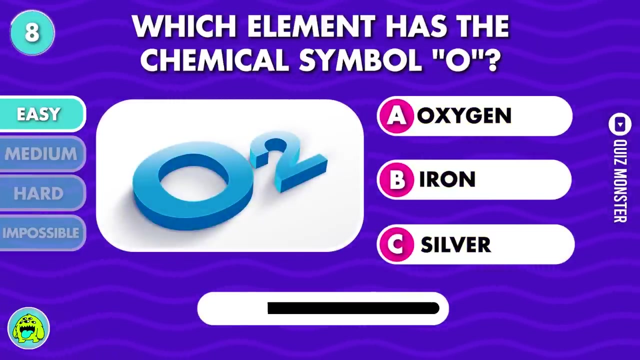 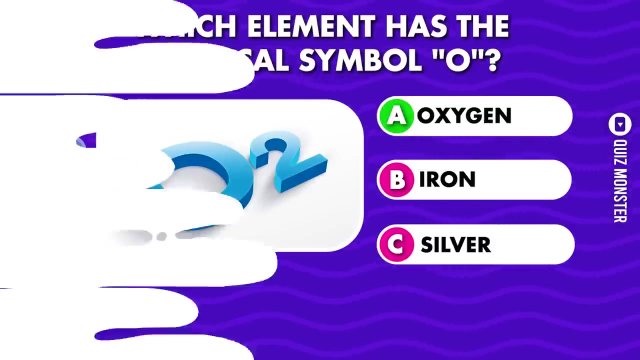 Day. Which animal is known for its black and white stripes? Zebra. What color is a ripe banana? Yellow. Which planet is known as the Red Planet, Mars? Which element has the chemical symbol O, Oxygen? What is the main ingredient in a burger? 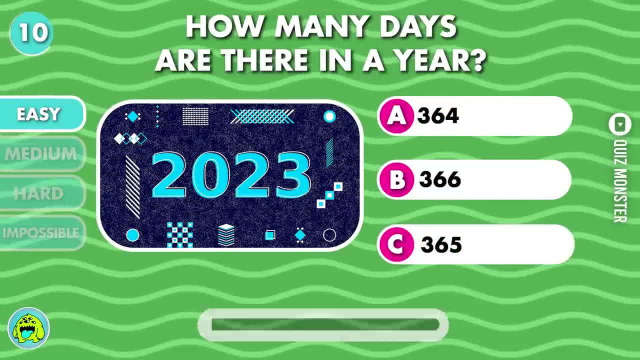 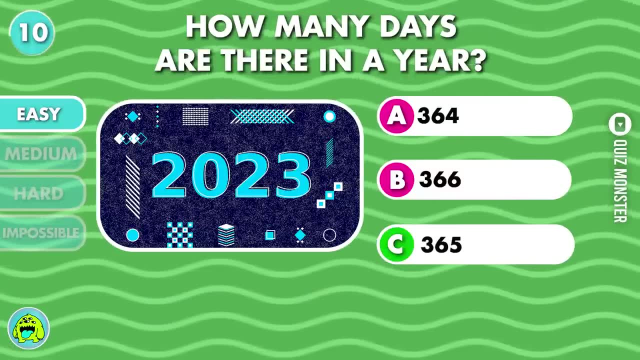 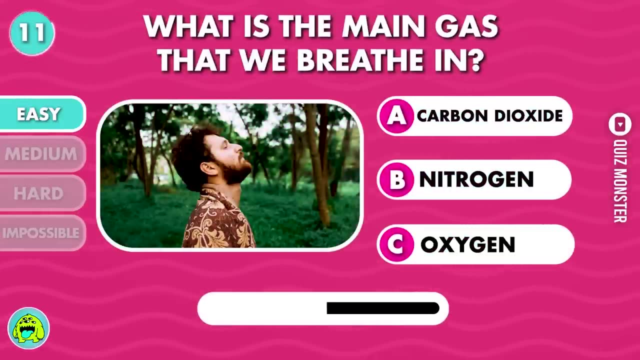 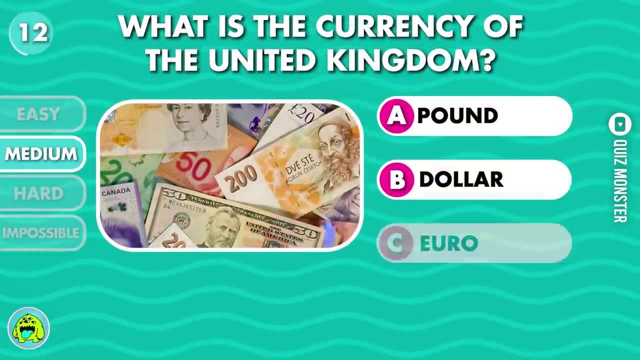 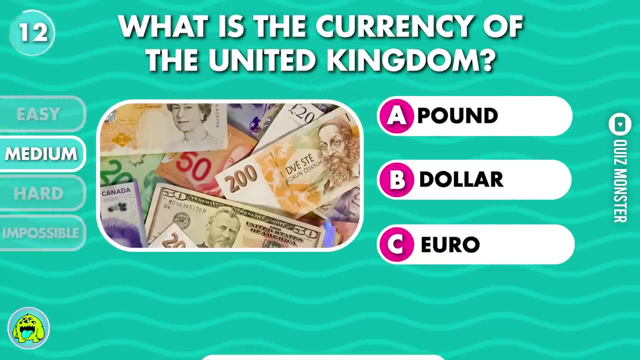 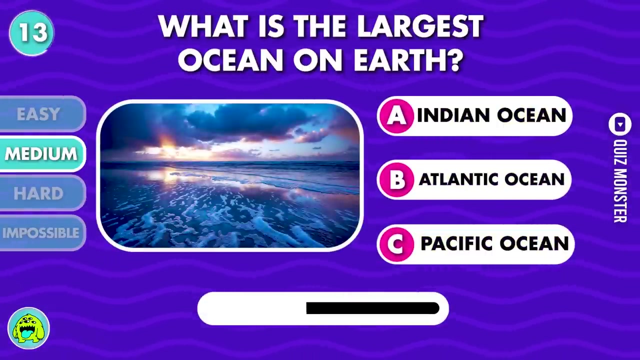 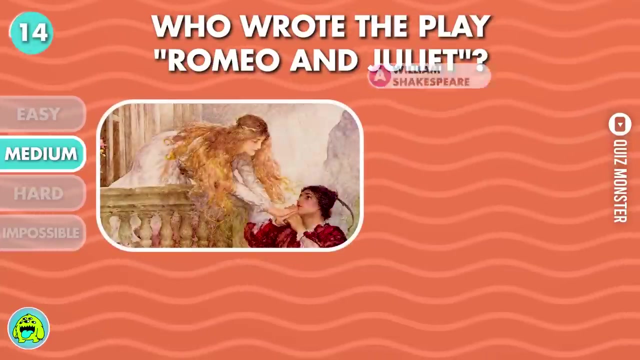 Beef. How many days are there in a year? 365!. What is the main gas that we breathe in? Oxygen. What is the currency of the United Kingdom- Pound. What is the largest ocean on Earth? Pacific Ocean. Who wrote the play Romeo and Juliet? 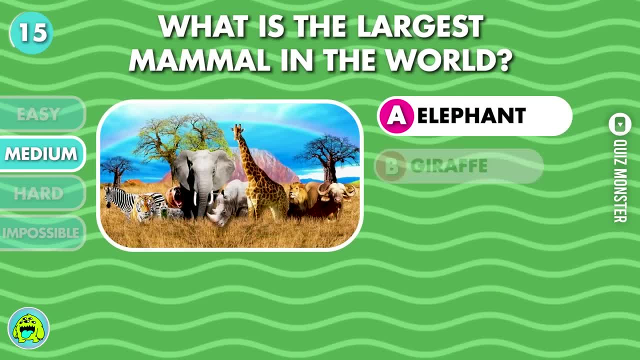 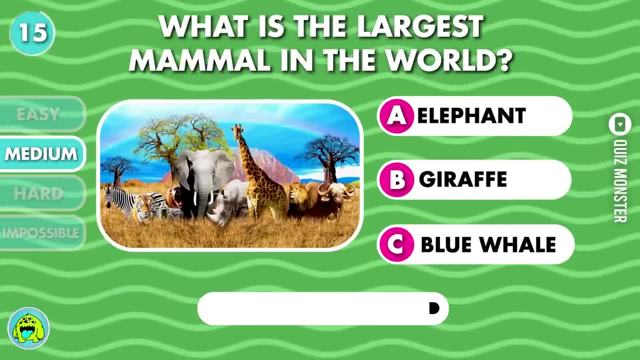 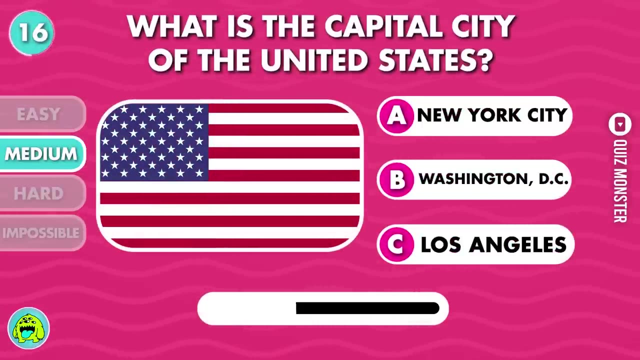 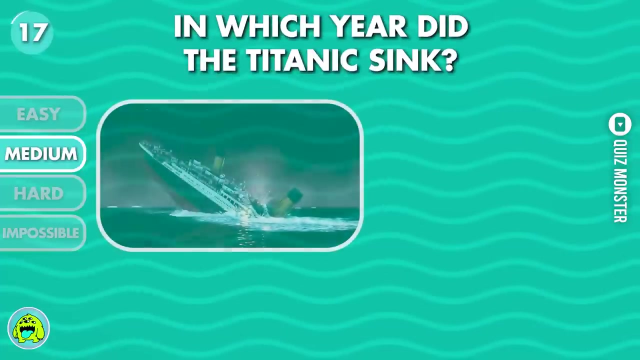 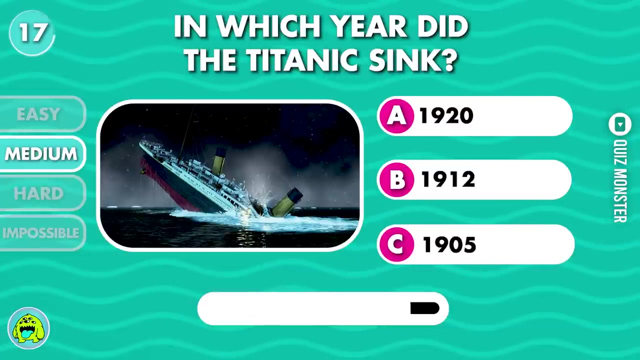 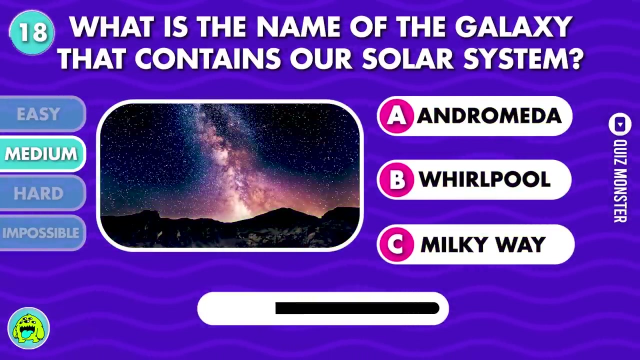 William Shakespeare. What is the largest mammal in the world? Blue Whale. What is the capital city of the United States, Washington DC. In which year did the Titanic sink? NASA, 1912!. What is the name of the galaxy that contains our solar system? 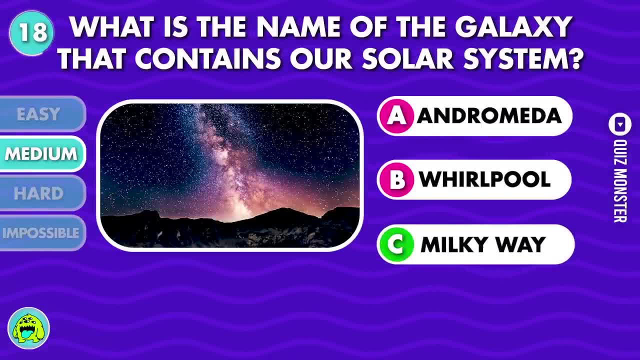 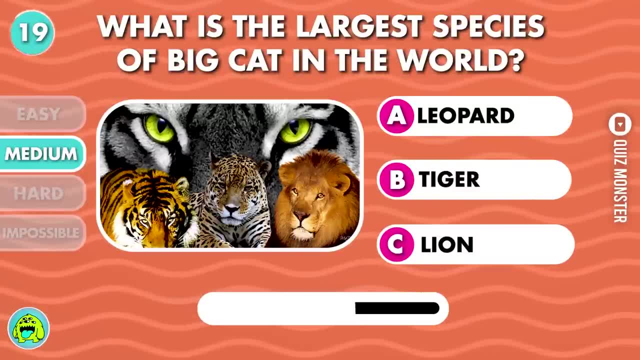 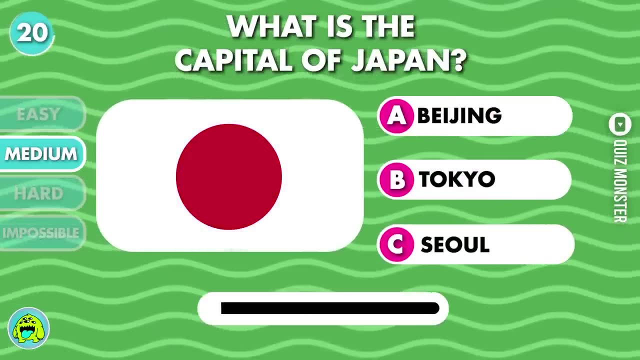 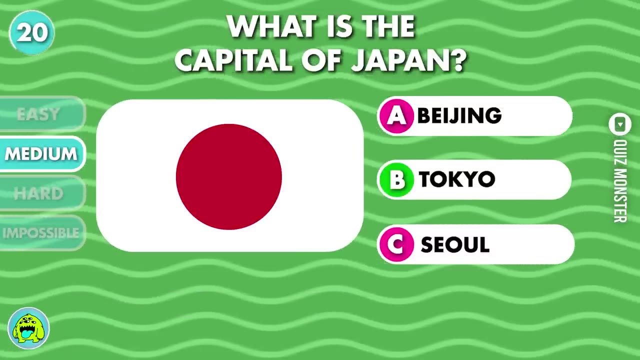 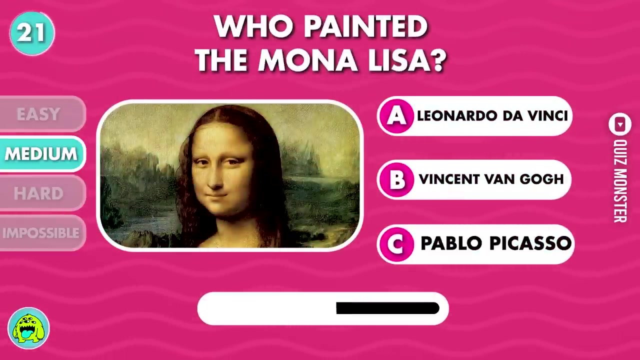 New York. What is the name of the largest object in the universe- Milky Way. What is the largest species of big cat in the world- Tiger. What is the capital of Japan, Tokyo. Who painted the Mona Lisa? Leonardo da Vinci? 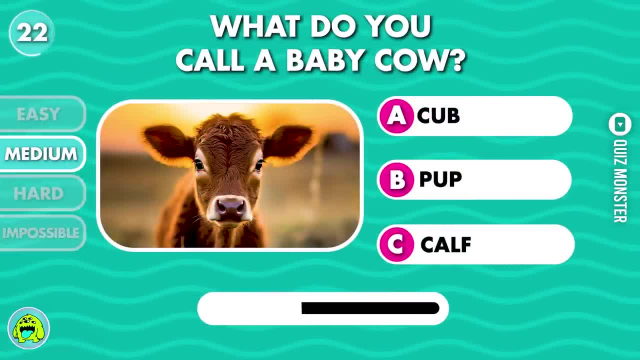 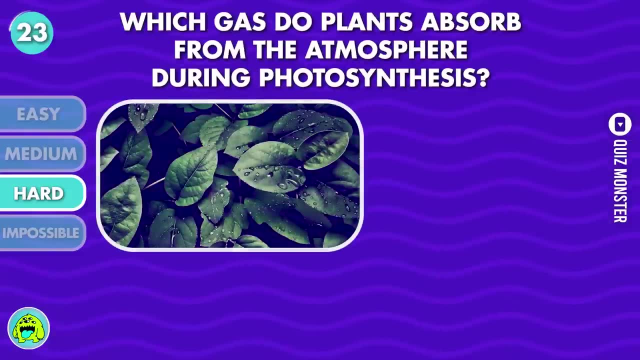 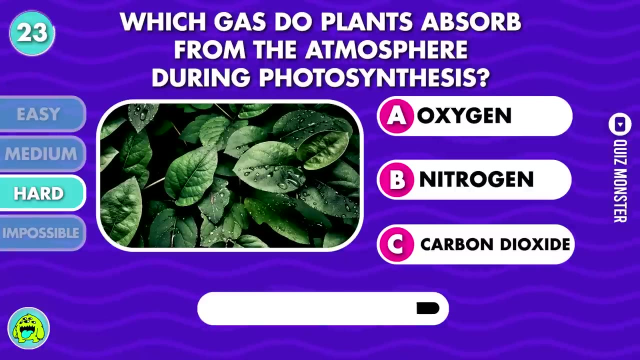 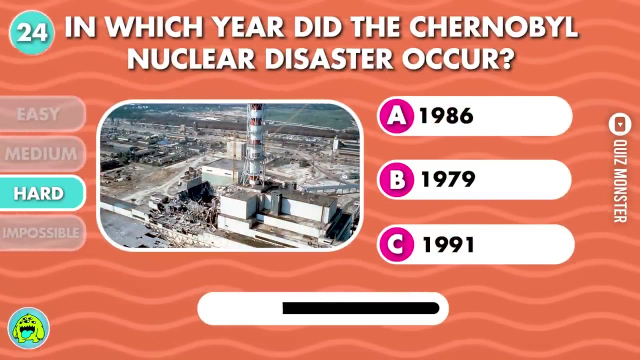 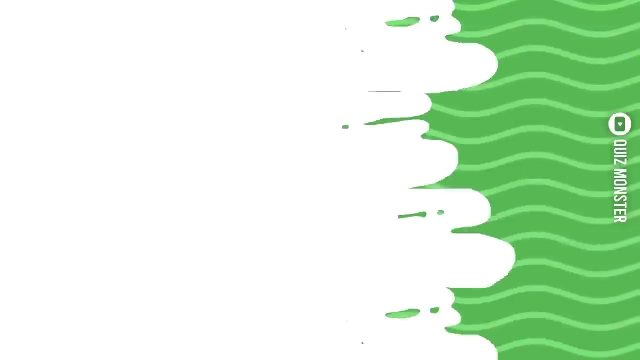 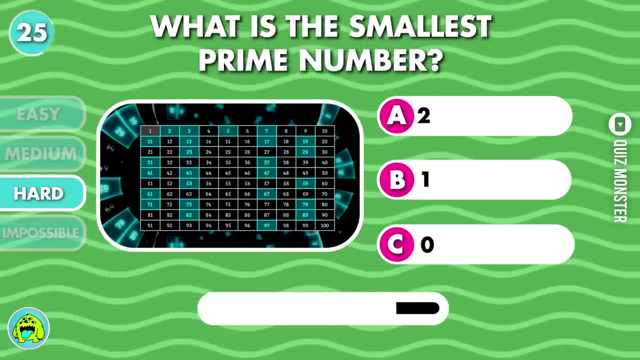 What do you call a baby cow, Calf? Which gas do plants absorb from the atmosphere during photosynthesis? Carbon dioxide. In which year did the Chernobyl nuclear disaster occur? 1986.. What is the smallest prime? number Two: 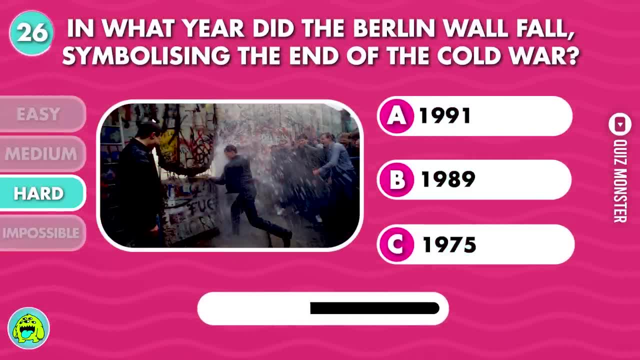 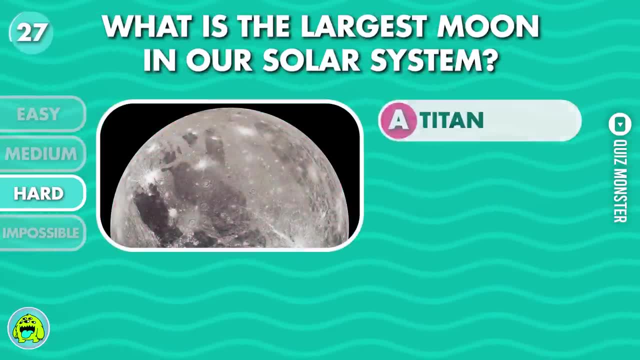 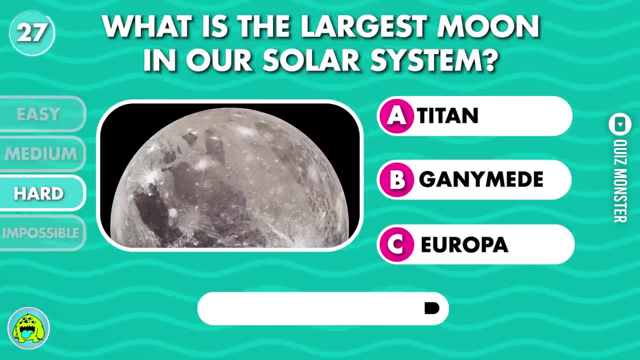 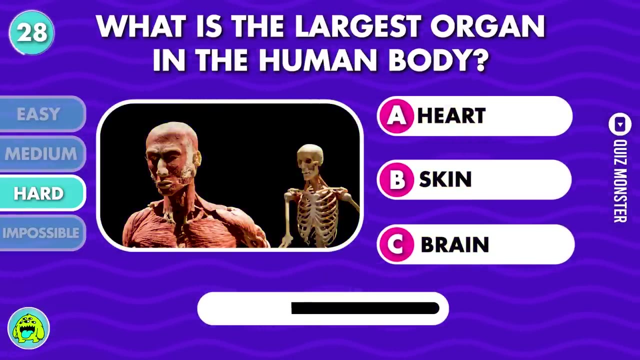 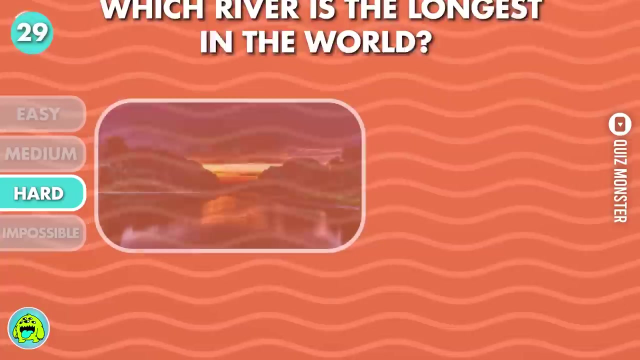 In what year did the Berlin Wall fall, symbolizing the end of the Cold War? 1989.. What is the largest moon in our solar system- Ganymede. What is the largest organ in the human body- Skin? Which river is the longest in the world? 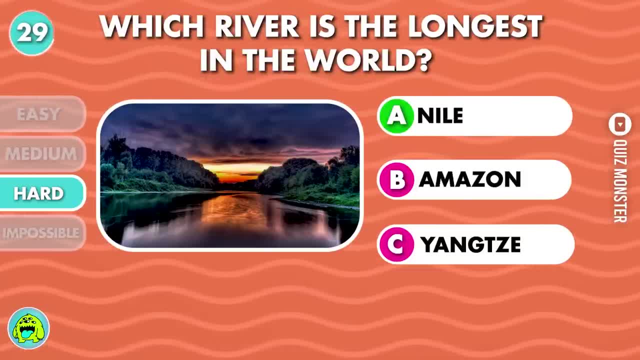 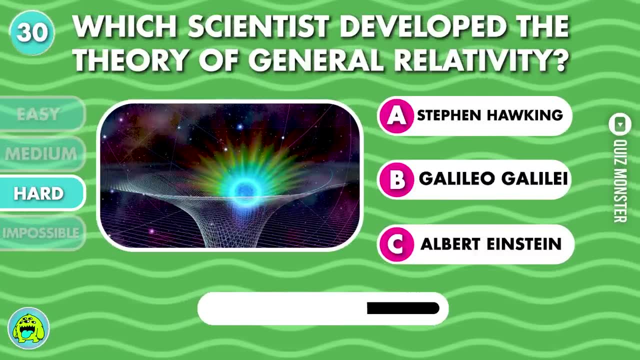 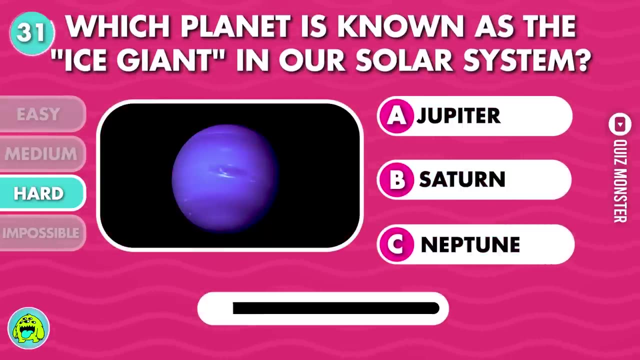 The river Nile. Which river is the longest in the water? The river Nile. Which scientist developed the theory of general relativity? Robert Einstein. Which planet is known as the ice giant in our solar system? Neptune. Which legend says that Another Planet I thought is only one? 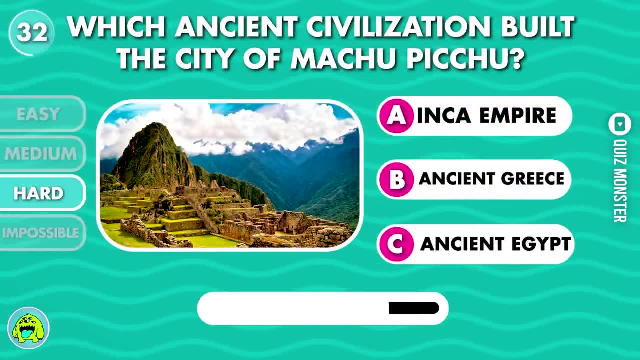 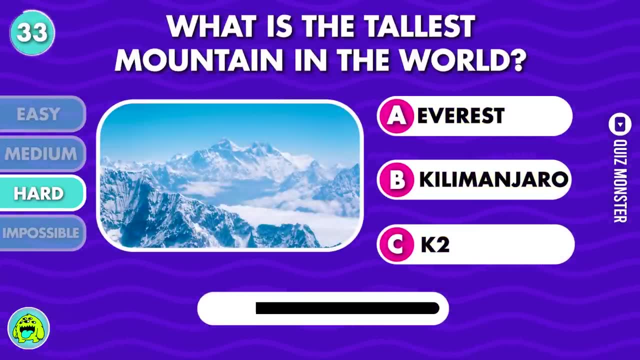 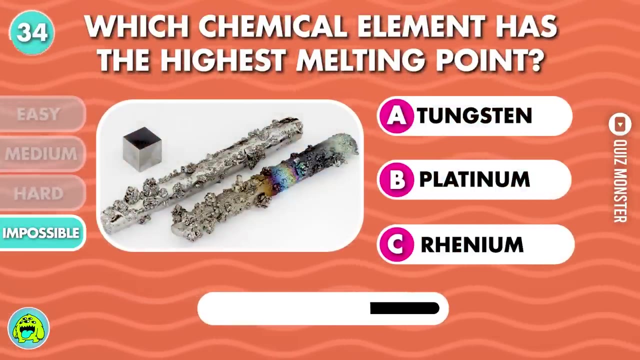 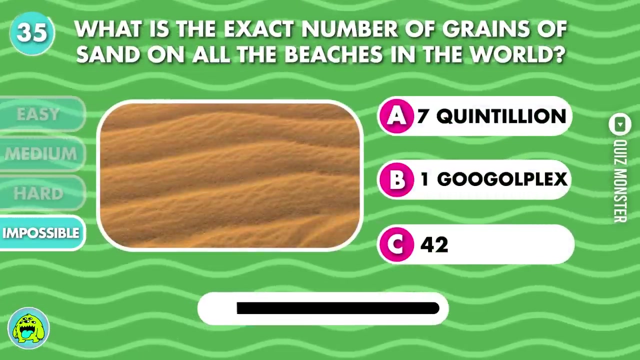 built the city of Machu Picchu, Inca Empire. What is the tallest mountain in the world- Everest. Which chemical element has the highest melting point- Tungsten. What is the exact number of grains of sand on all the beaches in the world? 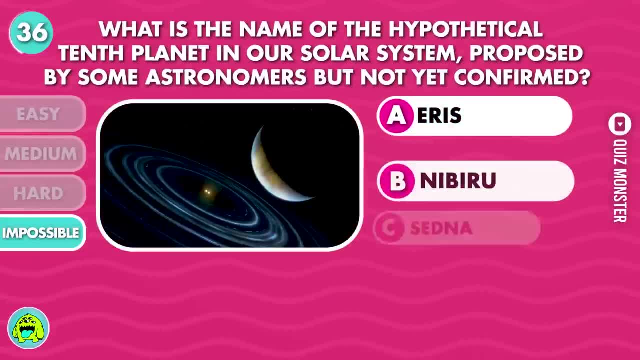 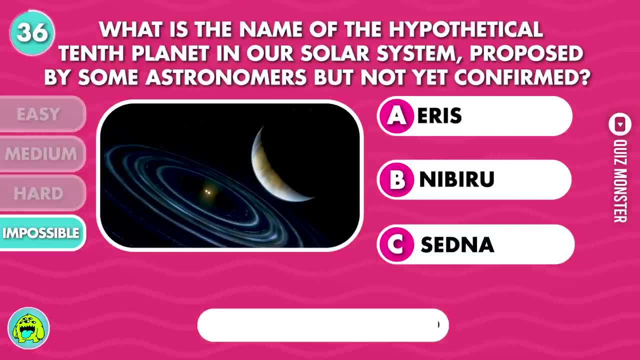 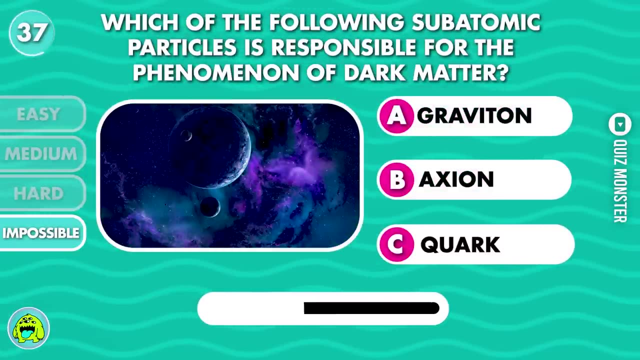 One googolplex. What is the name of the hypothetical 10th planet in our solar system proposed by some astronomers but not yet confirmed- Nibiru? Which of the following subatomic particles is responsible for the phenomenon of dark matter Axis? 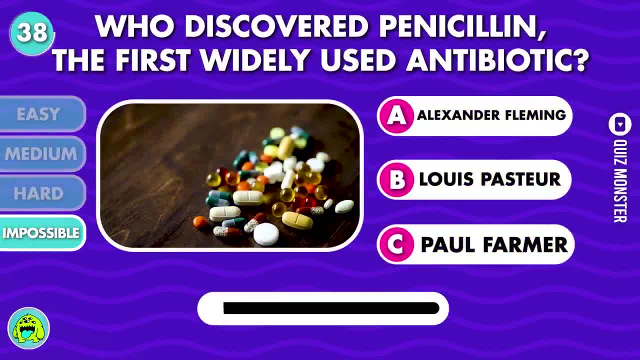 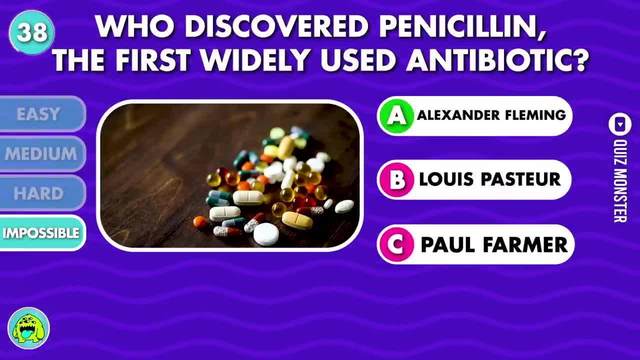 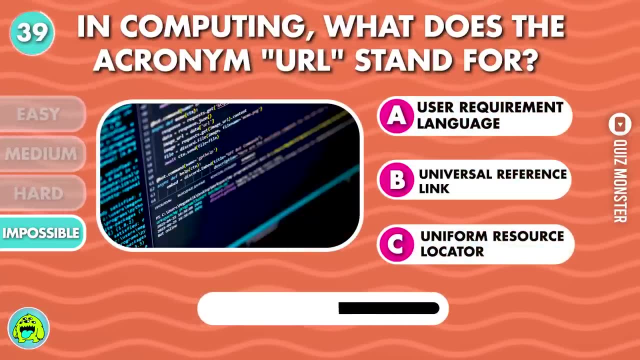 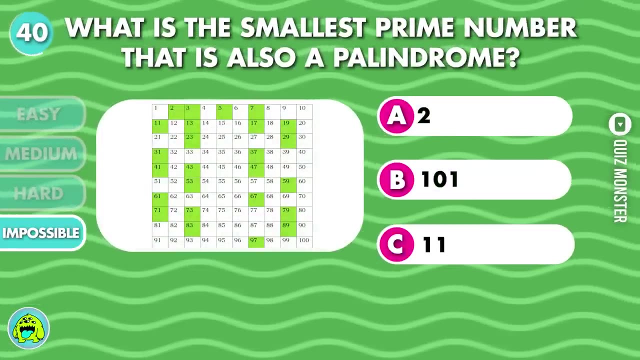 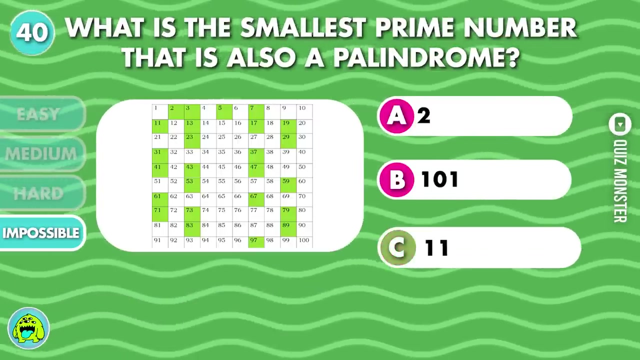 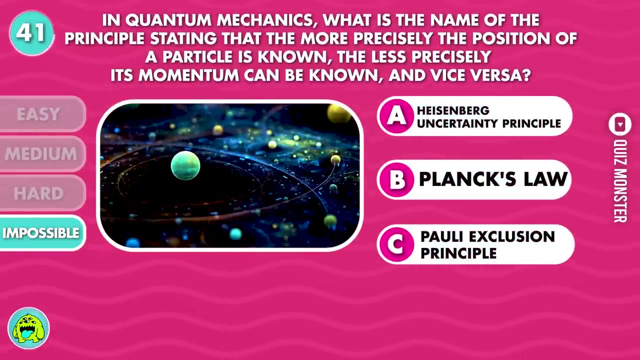 Who discovered penicillin, the first widely used antibiotic? Alexander Fleming. In computing, what does the acronym URL stand for? Uniform Resource Locator. What is the smallest prime number? that is also a palindrome, 11.. In quantum mechanics, what is the name of the principle stating that the more precisely the position of a particle is known, the less precisely its momentum can be known, and vice versa? 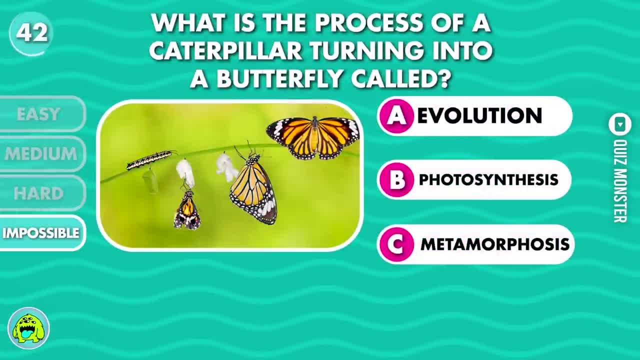 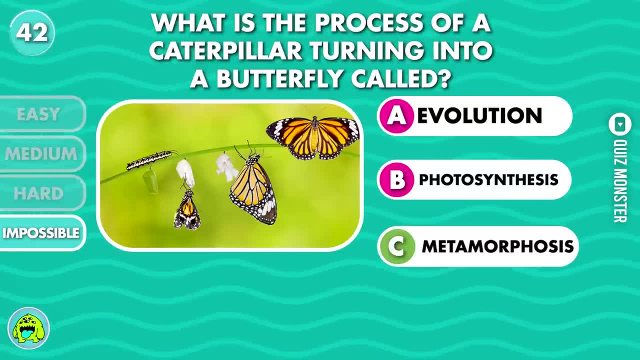 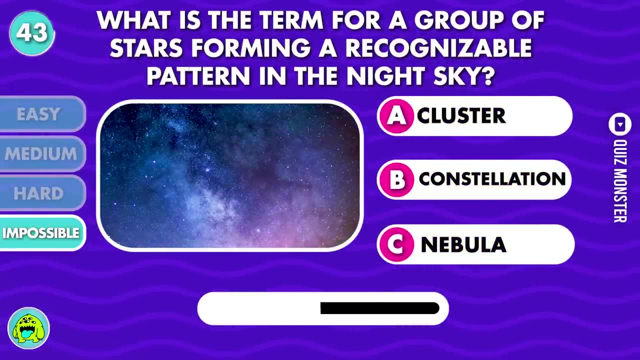 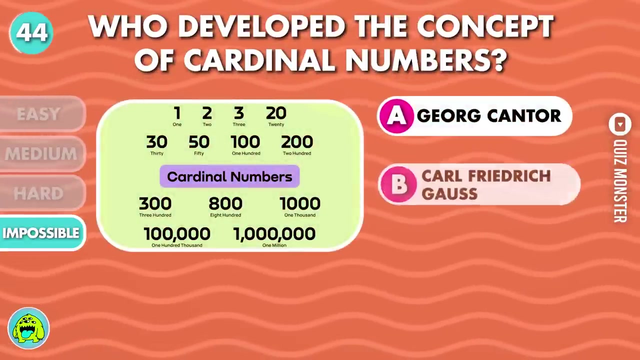 Heisenberg Uncertainty Principle. What is the process of a caterpillar turning into a butterfly called Metamorphosis? What is the term for a group of stars forming a recognizable pattern in the night sky Constellation? Who developed the concept of cardinal numbers? 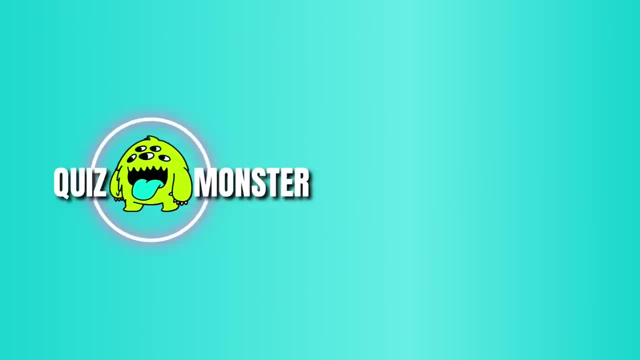 Georg Cantor, How many did you get? Comment down below and make sure to like and subscribe.